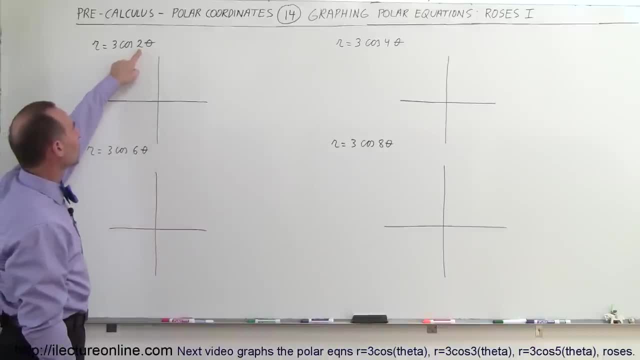 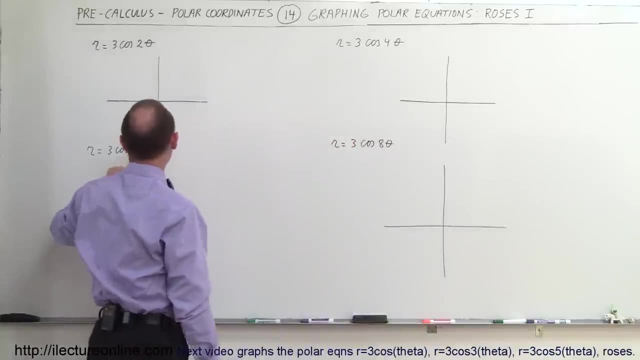 The way to work, that is, the number of leaves you end up with will be twice the number that you see here. So this will end up with four leaves, this one will end up with eight leaves, this one will end up with 12 leaves and this one will end up with 16 leaves. So that's how you determine and where the leaves. 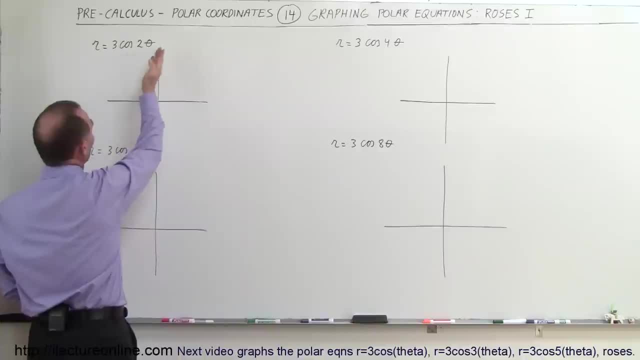 where the direction of the leaves will be well with the cosine of the function. remember, when the angle is zero, the cosine of the function is zero, So r would be equal to three in that case. so for a zero angle, the first leaf for the cosine will be in the 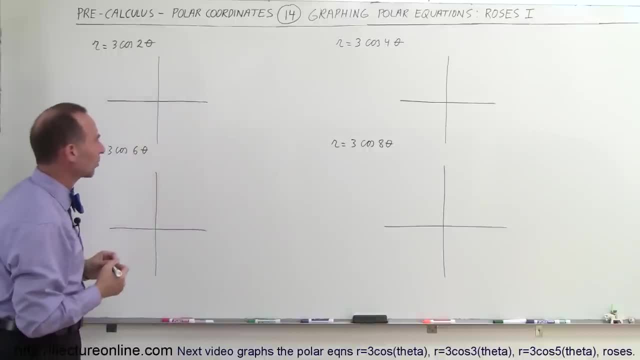 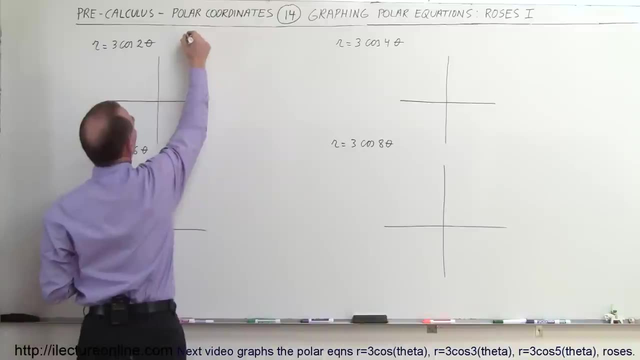 positive x direction or the to the right in the horizontal direction, And the number of leaves you're going to have is simply going to be twice the number here. so what you're going to do is you're going to take 360 degrees and divide it by twice that number two. 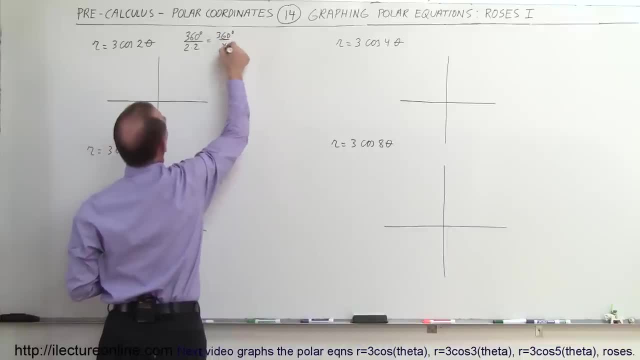 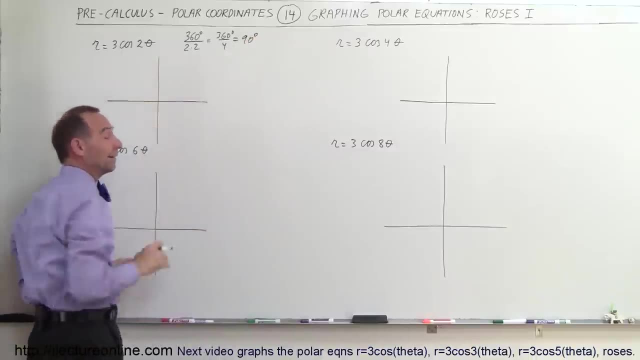 times two, which is 360 degrees. divided by four, which is 90 degrees, That means you're going to have a leaf every 90 degrees. so we're going to have one leaf every 90 degrees. That means you have one leaf here, one here, one there, one there, and that's how. 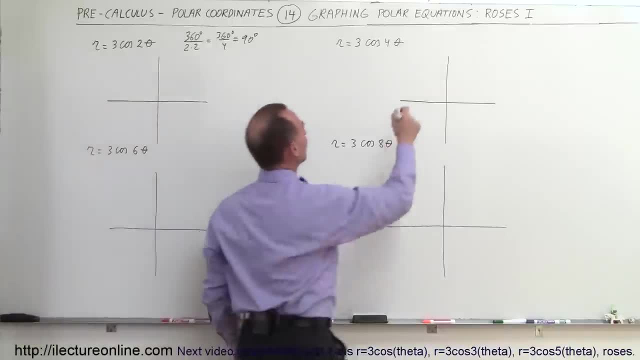 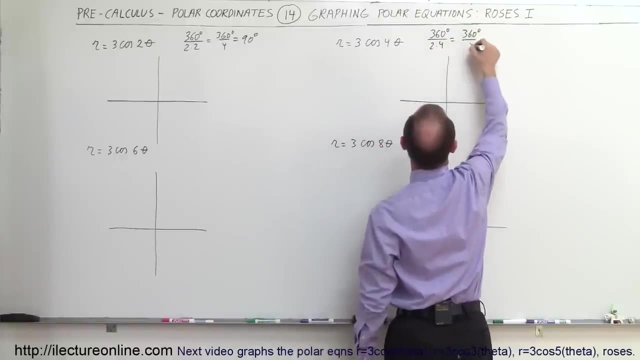 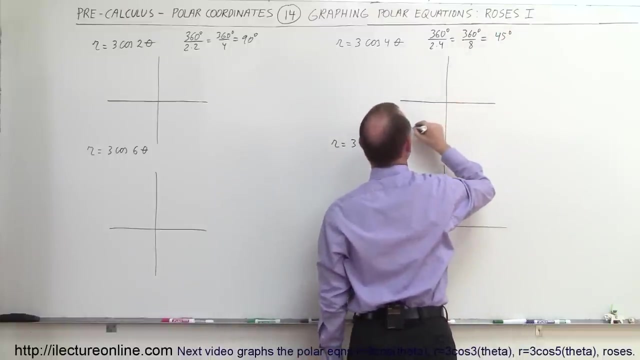 it's done So on. r equals three times the cosine of four theta. what you do here is you take 360 degrees divided by two times four, which is 360 degrees divided by eight. and, of course, 360 degrees divided by 8 is 45 degrees, which means you're going to have a leaf every 45 degrees. So we need 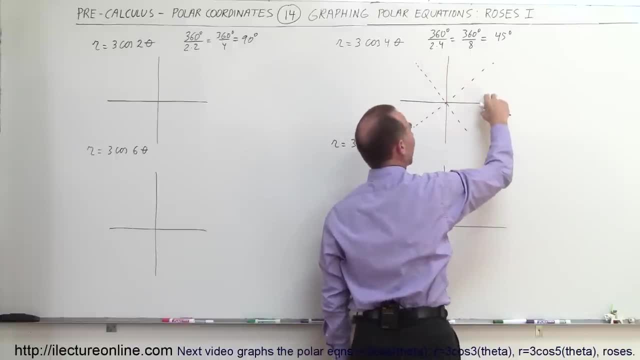 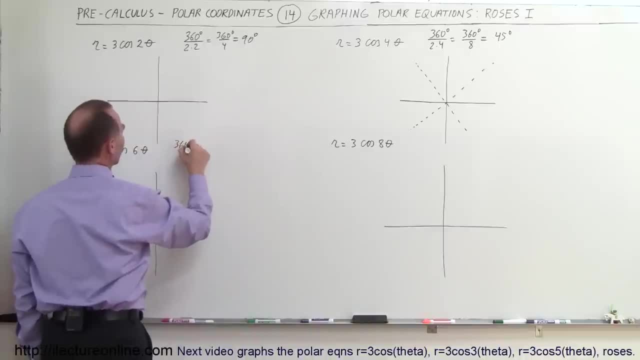 coming over here, you can say that you're going to have 360 degrees divided by two times six, which is 360 degrees divided by 12, which is equal to 30 degrees. that means you're going to have a leaf every 30 degrees. so we're going to draw those lines, so we're going to draw a line in this. 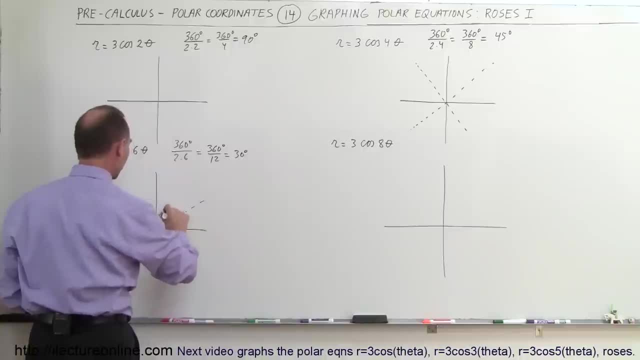 direction that's 30 degrees away from here, draw another one in 60 degrees, of course, we have one at 90 degrees. so we continue in this direction, continues this direction. we do the same over here, we do the same over here, and then we continue on this way and continue down this way, so that 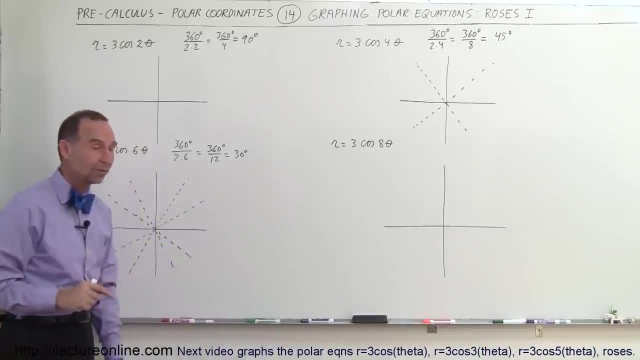 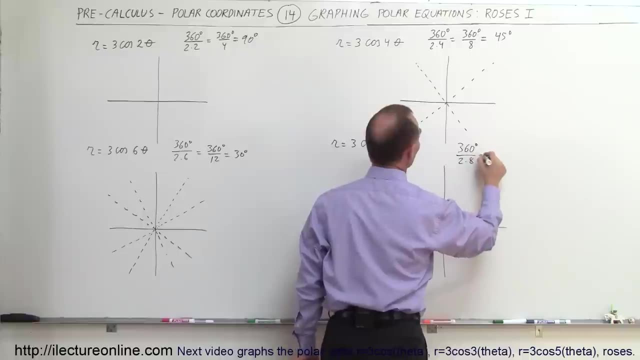 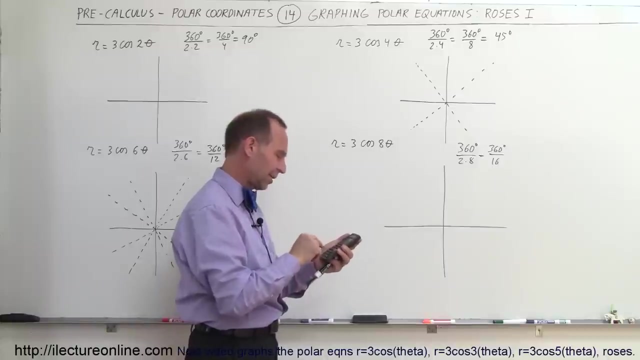 means you're going to have 12 leaves, one around each one of those lines, and finally we come over here. we can say that we take 360 degrees and divided by two times eight, which is 360 degrees divided by 16. and let's make sure i get that right: 360 divided by 16. 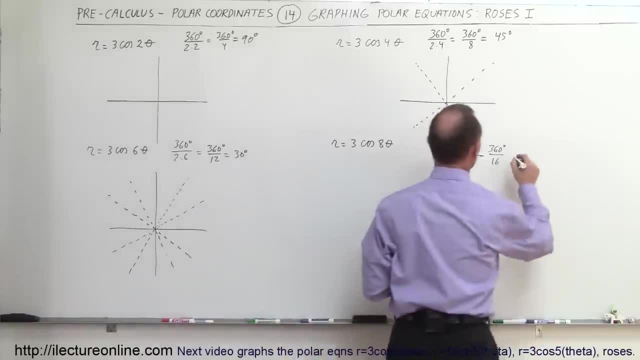 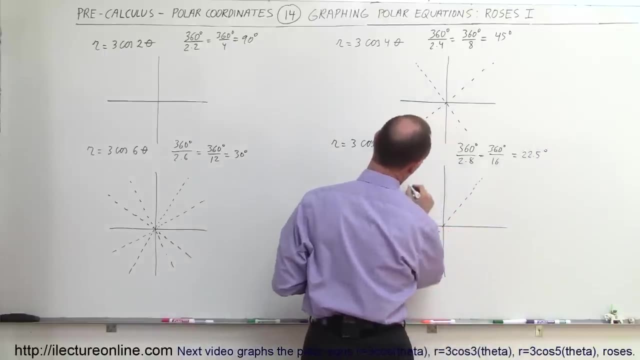 you, that would be every 22 and a half degrees. so that's equal to 22.5 degrees. so let's first put in the diagonals like this: this is 45 degrees this way, 45 degrees this way. and then we split each one, each one of them, up in 22 and a half degree lines. this way, 22 and a half degree lines. 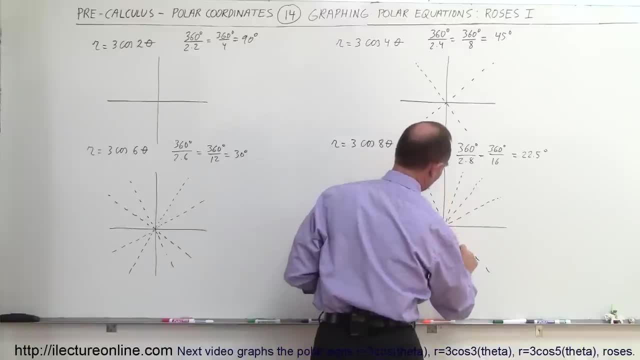 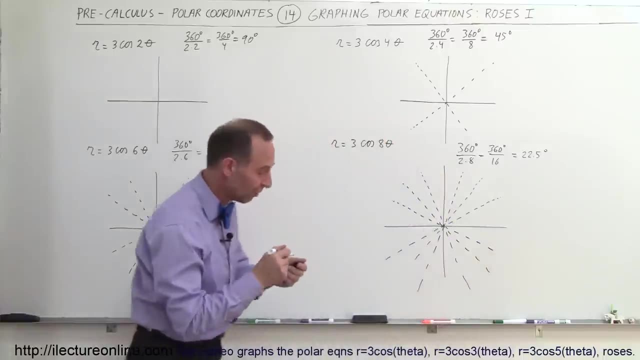 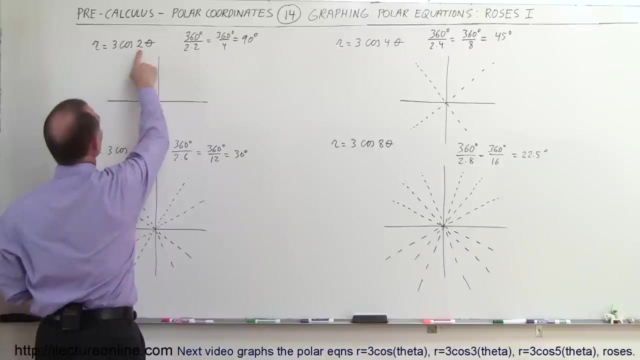 this way: a 22 and a half degree line in this direction and a 22 and a half degree line in this direction. so now we have 16 of these lines. each one will have a leaf of the graph on it, so let's try this one first. again, when theta equals zero, cosine of zero, zero, so three. 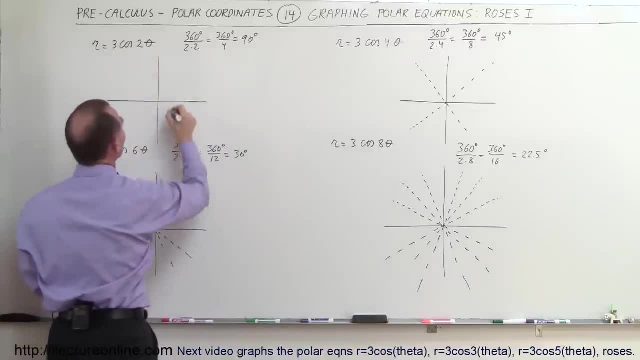 times- oh, i'm sorry- cosine of zero is one. three times one is three. so go one, two, three, and so we have the top of the leaf. and what happens then is the leaf will look like this: come through the origin. we'll go like this, and again it'll hit the point. r equals three. we'll come like this: 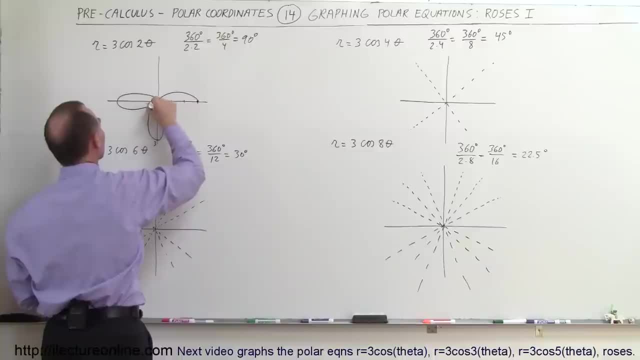 and we'll go around this graph. we'll come like this and we'll go around that graph and then come back this way: go around this graph and there you go. that's the graph representing. r equals three times the cosine of two theta, where the distance to the top of each leaf is equal to three of. 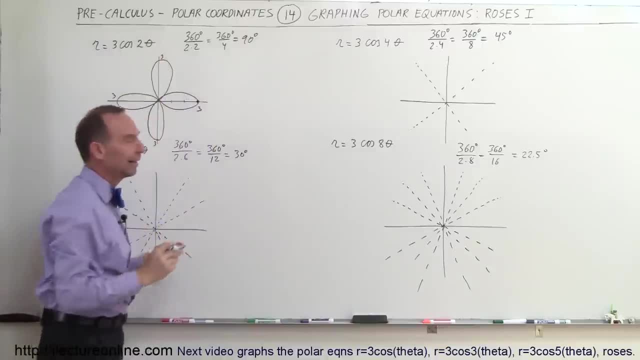 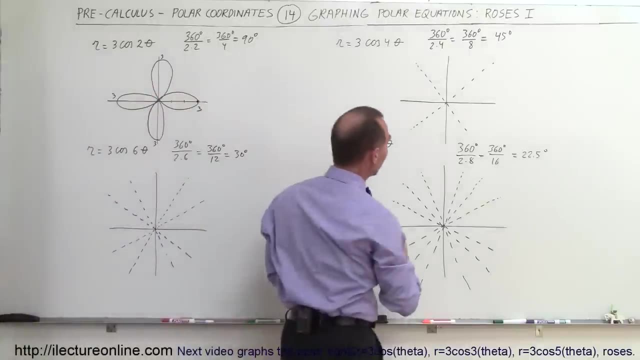 course, if this was a four or five, then of course the leaves would be bigger. that's how we do that. so here we do the same thing. now, instead of only having four leaves, there will have eight leaves. so again, starting with. theta equals zero, cosine of zero is one, so r equals three. so we start at. 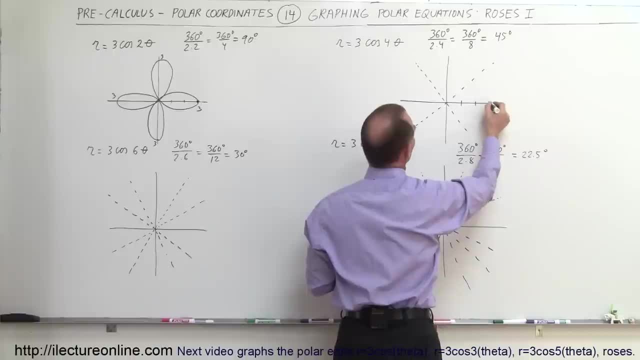 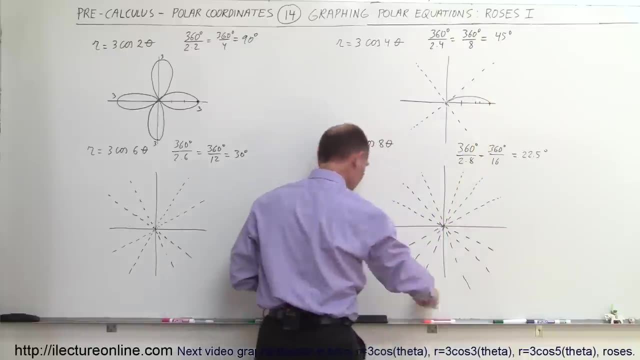 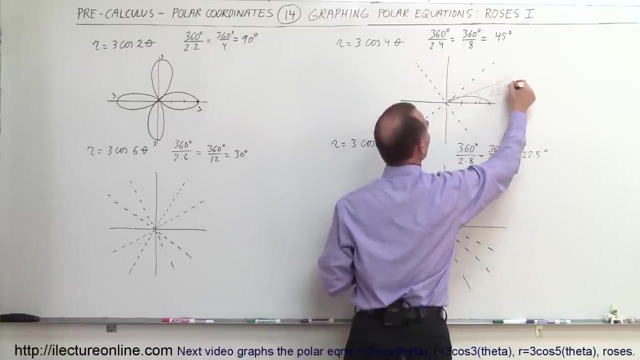 this point, one, two, three over here and notice that this will go like this. so at this point we've traveled through an angle of 22 and a half degrees, so let me go ahead and use a different color to denote that. so when we've moved to an angle of 22 and a half degrees, 22.5 degrees, 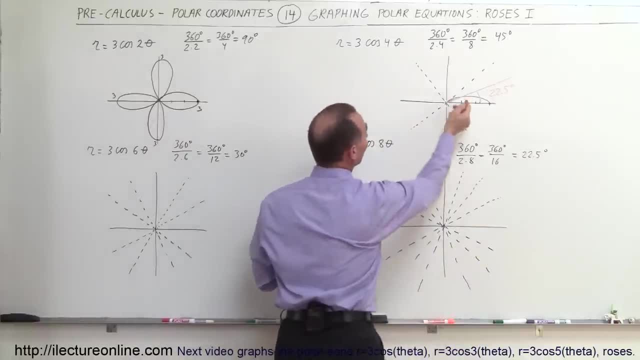 hope you can see that it's not very bright. at that point we come back to zero, because four times 22 and a half degrees is 90 degrees and the cost of 90 degrees is zero. so r should be be zero. so that would be the first portion of the first leaf. Now what happens when? 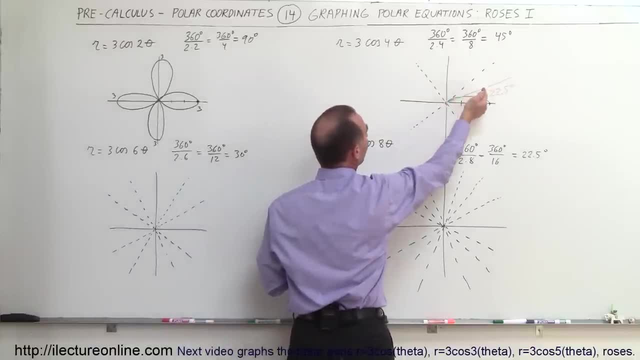 we go to the next 22.5 degrees. So when we get to 45 degrees we go back to zero, because four times- actually four times 45 degrees is 180 degrees. that would be minus one. so when we get to a 45 degree angle, we're at negative one times three, which puts us right. 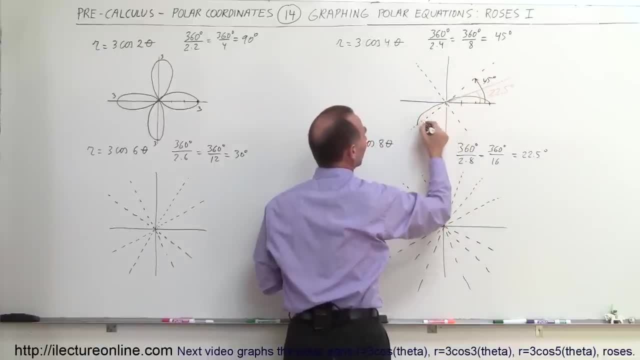 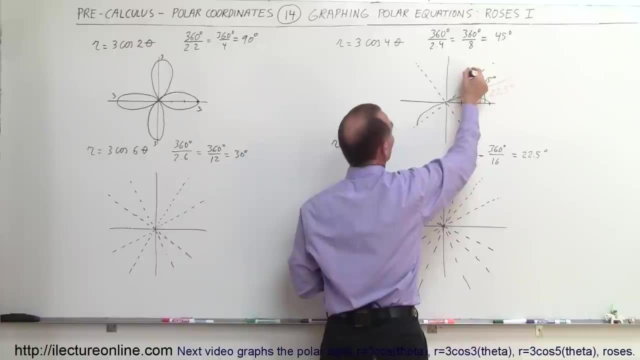 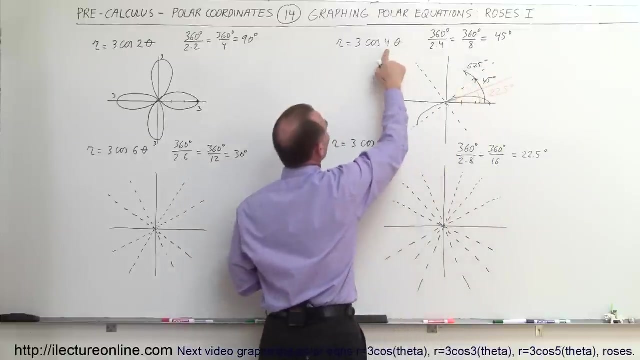 over here. so that means the curve continues and ends up over there at an angle of 45 degrees. So when we go another 22.5 degrees, so now we go to another, that would be 67.5 degrees. so we add another 22.5 degrees, then four times 67.5 degrees is 270 degrees. cosine: 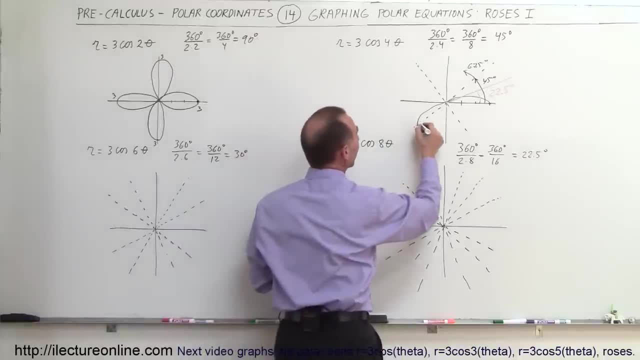 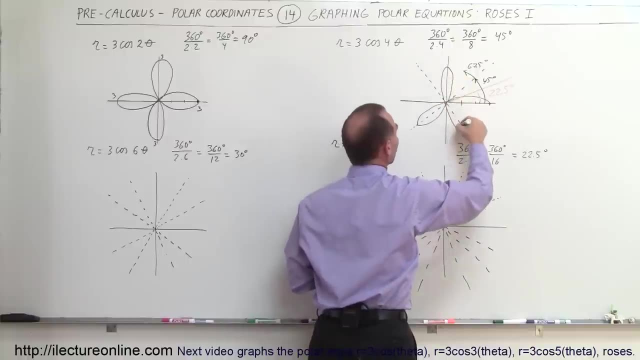 of 270 degrees is back to zero, so that means we come back over here. And so you can see, if you continue this pattern, then this pattern will look like this: come around, it'll look like this. come around, it'll look like this. come around, it'll look like this: 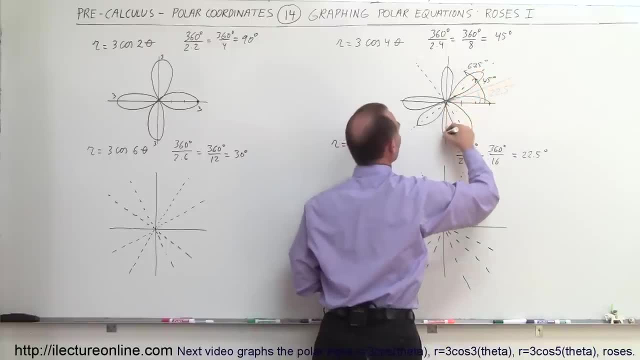 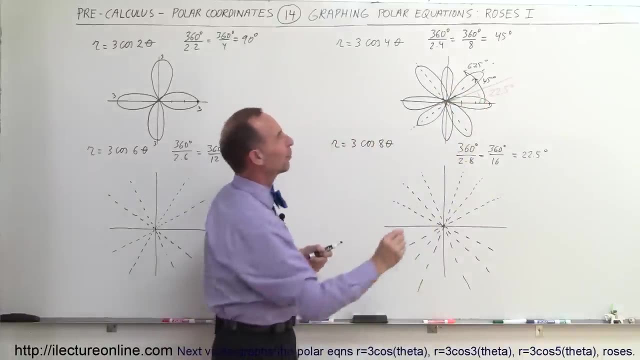 It looks like this, come around, this come around, like this, come around, and finally completes the circle like that. Now, to be accurate, of course, all the lines should go exactly to their origin. I didn't quite manage that, but at least you get the general. 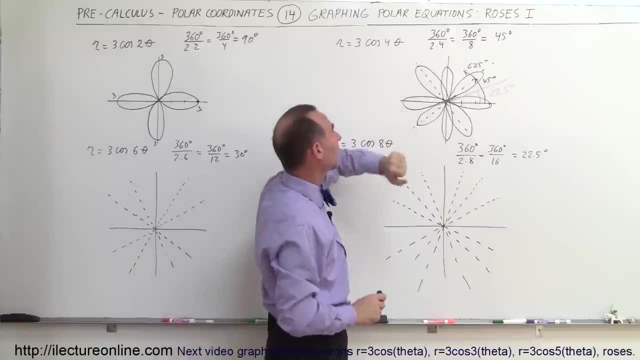 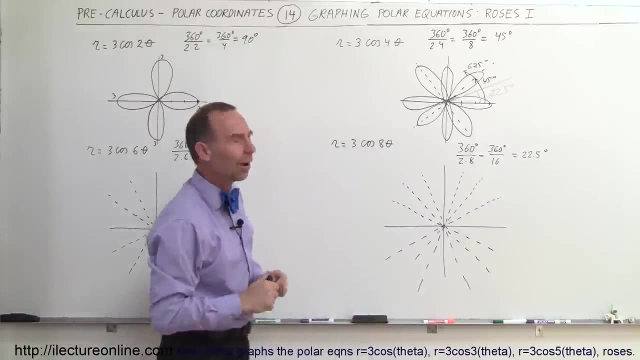 shape of what that looks like. when we have three times the cosine of four theta, You should have eight leaves. the distance to the edge of the leaf is three in each case. that's determined by this number and that's how we graph that. Alright to understand. 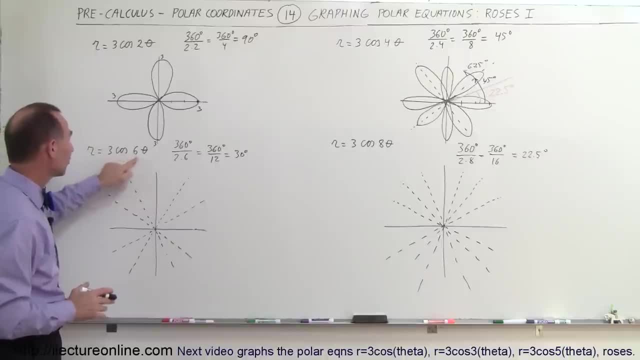 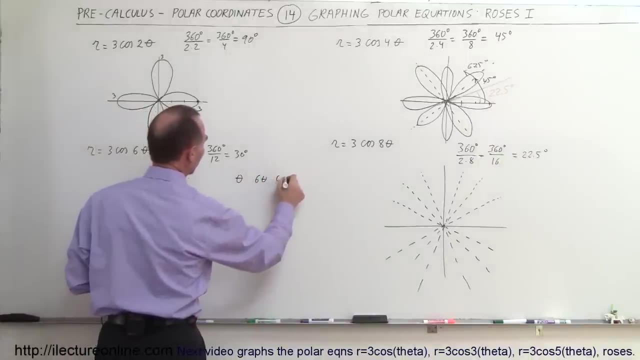 how to graph this one right here. r equals three times the cosine of six theta. it's probably a good idea to build a table of values, So let's try theta, six theta, the cosine of six theta, and see what we get. So, at zero degrees, of course, six times zero is still. 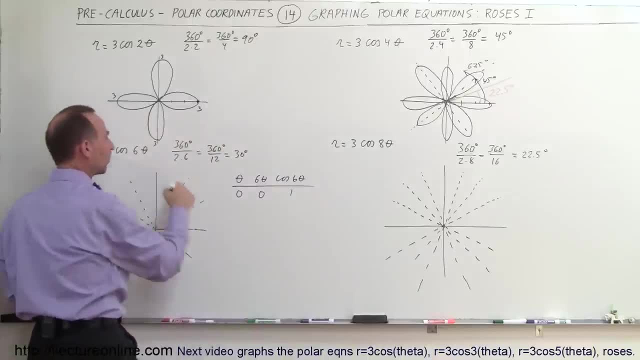 zero and the cosine of zero is one, And of course three times that would be. so three times the cosine of six theta, that would of course be three. Now let's move to an angle of fifteen degrees. If we go to an angle of fifteen degrees, three times the cosine of 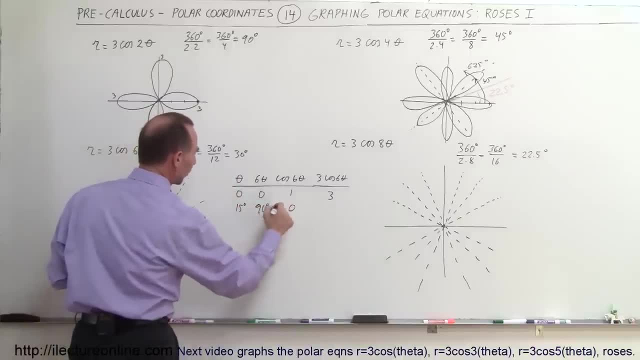 fifteen degrees. six times fifteen is ninety degrees. now we're back to cosine of nine is zero, and that would be zero If we now go to thirty degrees. thirty times six is one hundred and eighty degrees. the cosine of one hundred and eighty degrees minus one. 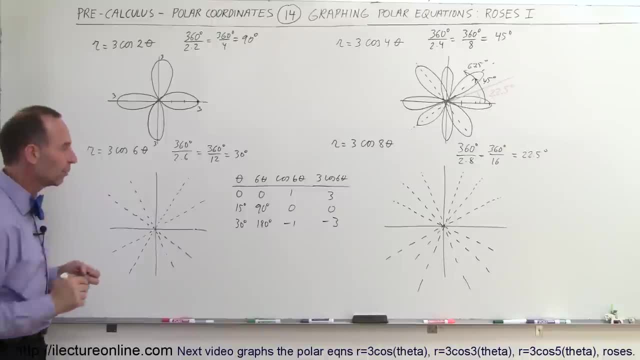 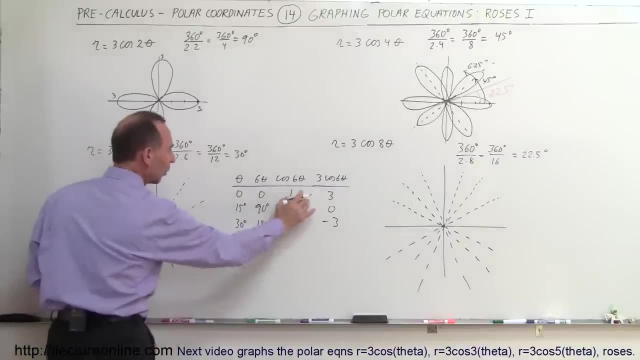 and that means we get minus three. And I think now you see the pattern of what's going to happen. So, at zero degrees, one, two, three- the graph is right there- three times one would be three right there At fifteen degrees if we go to an angle of fifteen degrees. 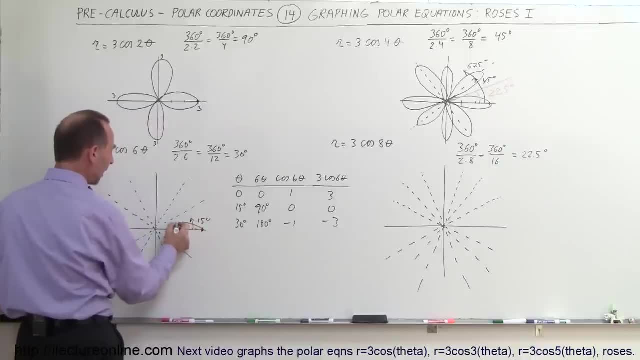 which is right here, that's an angle of fifteen degrees degrees. then we get back to zero. then if you go from 15 to 30 degrees- so now we go from 15 to 30 degrees, there's 30 degrees. that's the first line here. past the horizontal line, now 6 times 30 is. 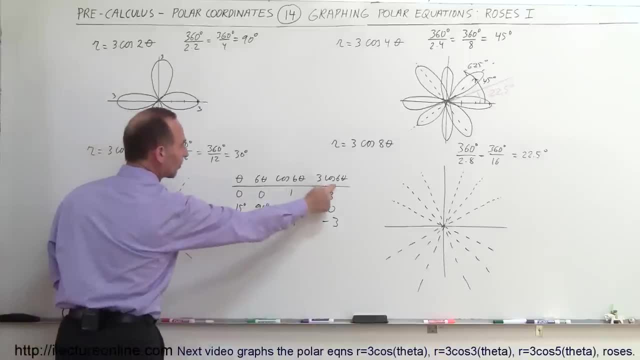 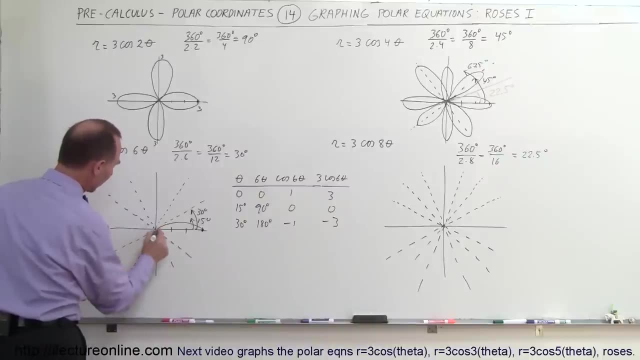 180. the cosine of 180 is minus 1 and therefore 3 times that would be minus 3, so we're pointing in this direction. we'll have an r value of minus 3, which puts us over here. so that means the leave continues on this way. it will then complete like this: so now we've gone through an angle of 45. 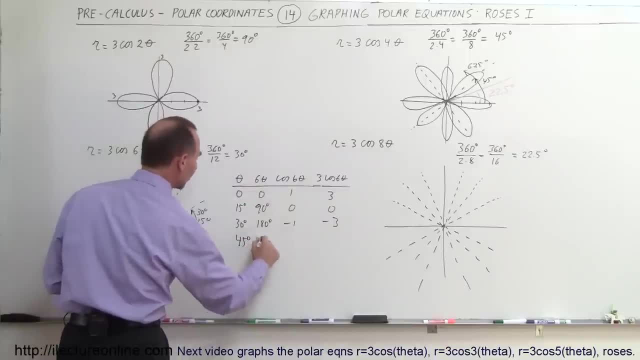 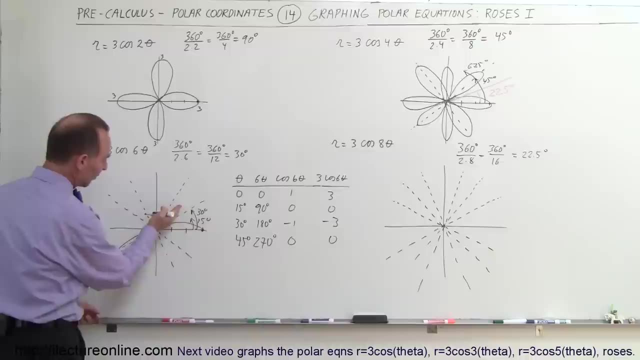 degrees, because 6 times 45 degrees is 270 degrees, which puts us back to cosine of 270 is zero, which makes this zero. so now we've moved to an angle of 45 degrees, which is right over here. we're back to zero. now, once we continue to the angle, we get to the next leaf right there, and then we come down. 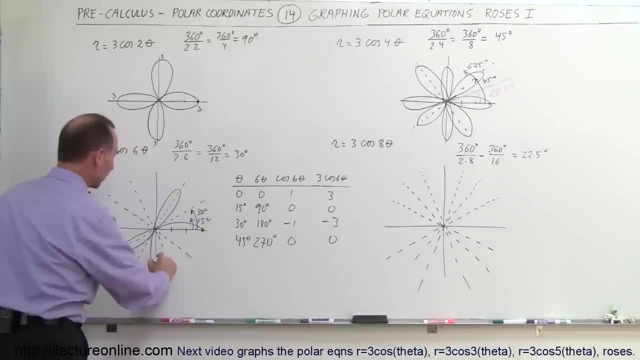 here, and then we go to the next leaf right here, you and we come this way: the next leaf right here and back down. and now we go to the next leaf right here and back down. the next leaf right here, back down, the next leaf right here, back down, the next leaf. 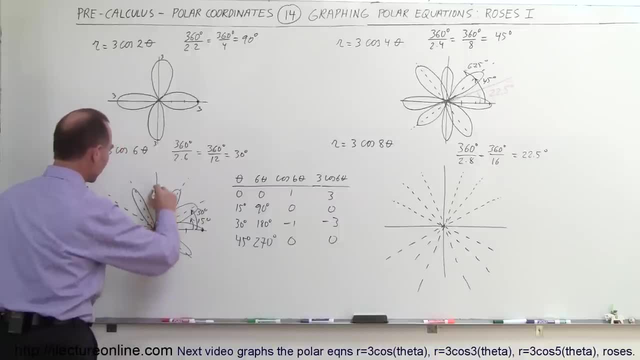 right there, back down the next leaf, right here, and you can see how that slowly works its way through this way and this way and finally we complete over here and that's what that graph will look like. That is a graph of r equals 3 cosine of 6, theta, and there should be 1,, 2,, 3, 4, 5, 6,, 7,, 8,, 9,, 10,, 11,, 12 leaves all the way around. 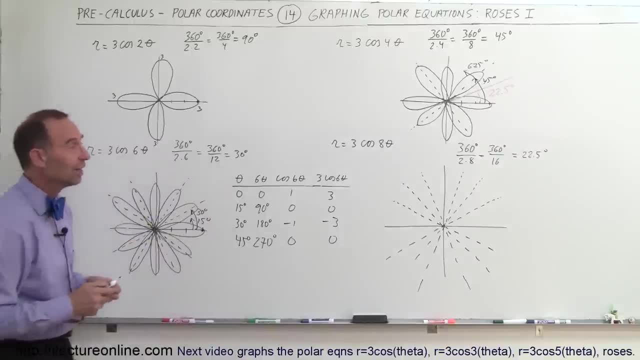 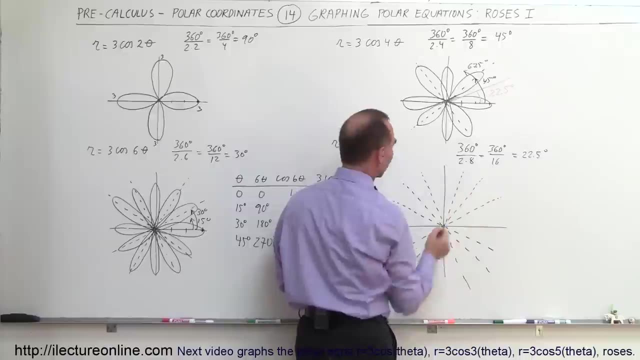 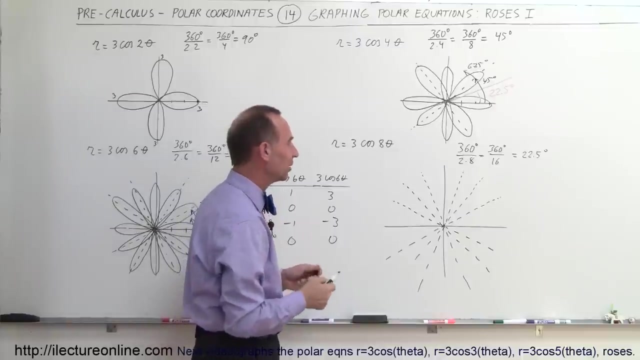 Wow, what do you think that one will look like? Same kind of thing. There we realize that every time we move through 22.5 degrees we go all the way from 0 to the next leaf. So you can see that 8 times 22.5 degrees would be 180 degrees. then we get to the negative value of the cosine. 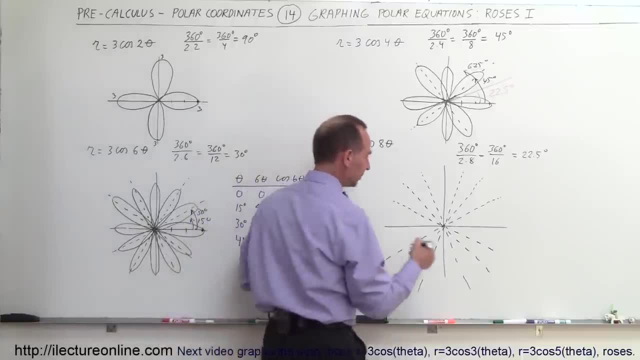 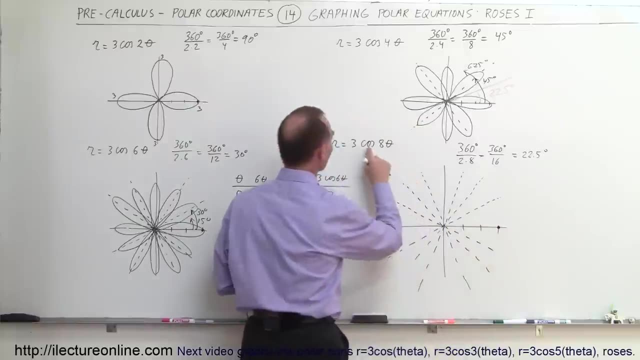 Well, let me show you. let me illustrate what that looks like Again. when the angle is 0 degrees, we have the maximum value. so cosine of 0 is 1, 3 times 1 gives us a value for 3, so that puts us at the end of the leaf, right there. 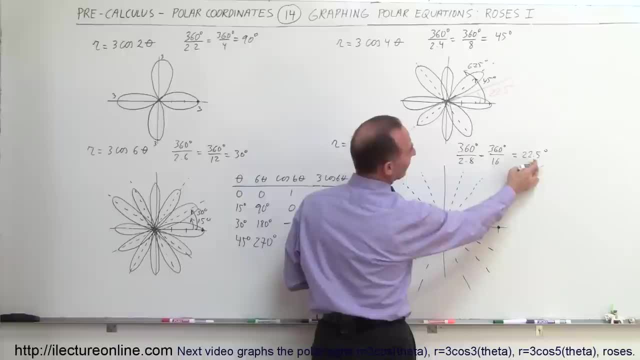 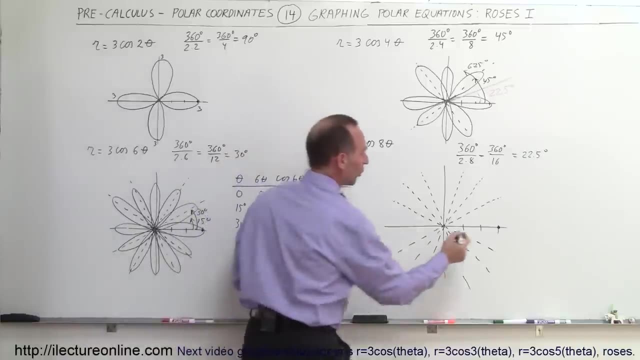 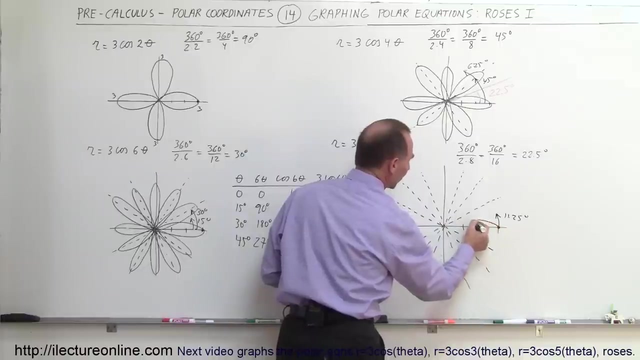 If we then move through an angle of 11.25 degrees, 8 times 11.25 degrees is 90 degrees. at 90 degrees the cosine goes to 0. So through an angle of 11.25 degrees we go from 3 all the way down to 0.. 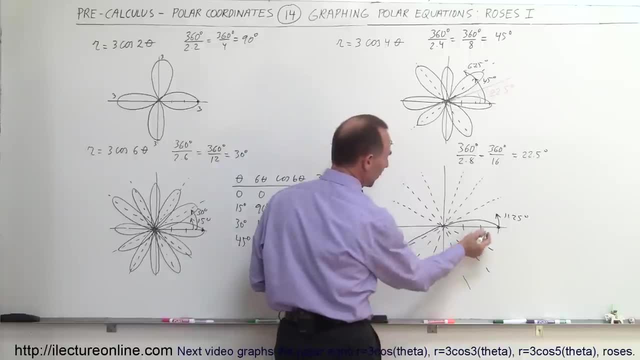 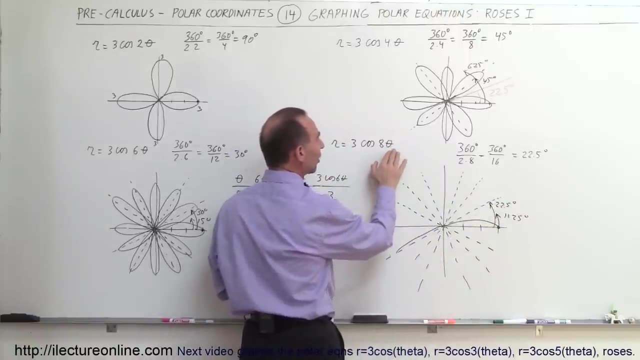 Then we get to the next leaf right here, and then, of course, when we move through an angle of 22.5 degrees, then you can see that 8 times 22.5 is 180, cosine of 180 is minus 1, so 3 times minus 1 is minus 3,. 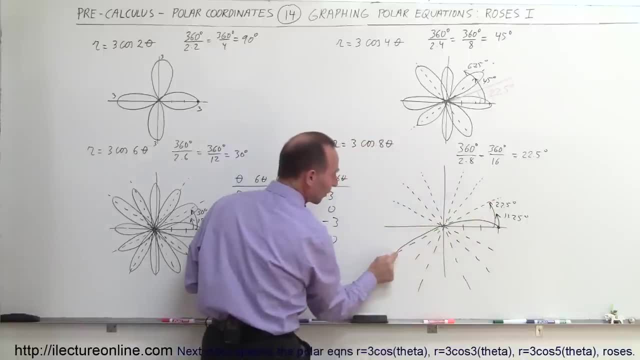 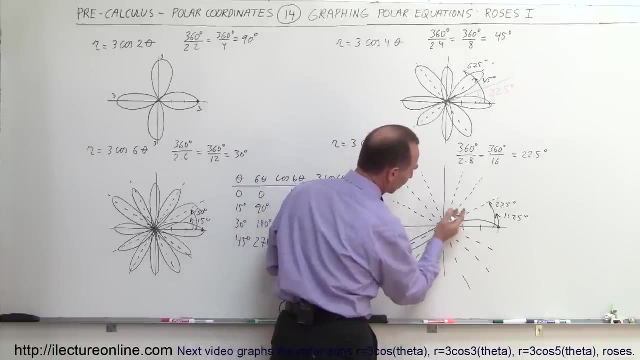 so when we are pointing in this direction, the value is minus 3, that's how we end up over here, And then you simply just go to the next leaf. Let me go back here and make that look particular in a minute, and this is how I do it with theínaon left. 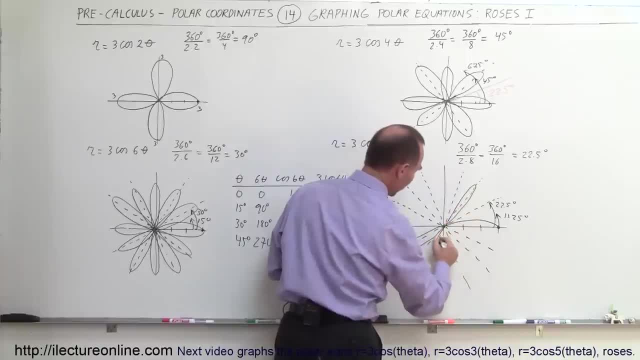 So this one looks exactly like this. So now we're going to go through this one right here and back down and this one right here and back down, and not to come around to this one and back down. so now we come around to this one.